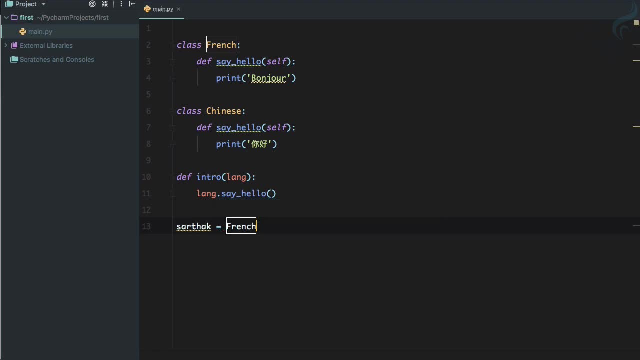 instance of French, and my name is Sarthak, so I speak French, but John is going to speak Chinese. so let's now see if we use the intro function- and I will pass Sarthak here- what will be the result? what function it is going to call Chinese or French. let's 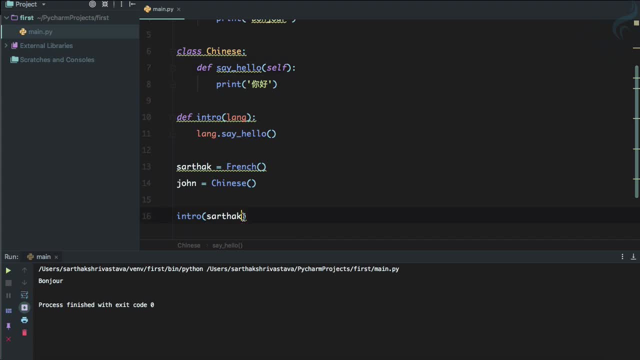 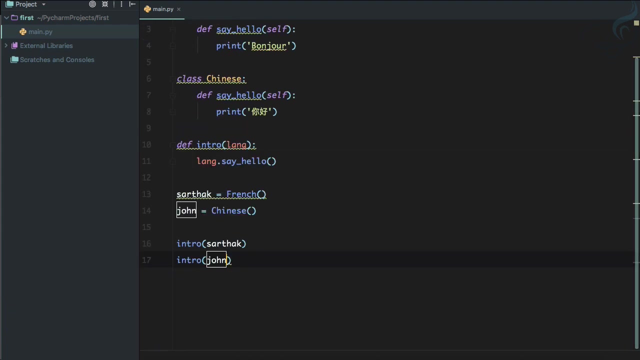 run it and yes, bonjour is there. and similarly, if we say intro for intro for John and now run, yes, you can say: you can see here, eha is there. so why is eha for John and bonjour for Sarthak? see, because John is an instance or John is an object of Chinese class. so this object go to intro function. 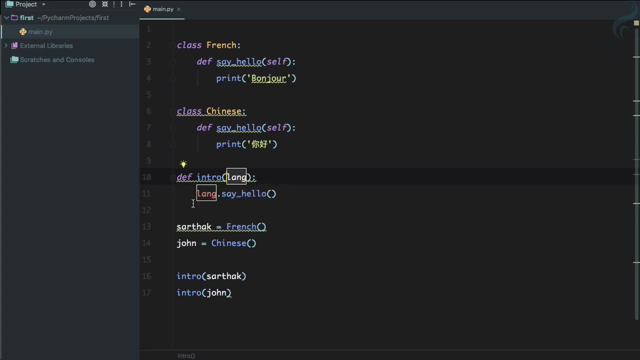 intro function, except that object and it will say object dot, say Hello. whatever is the object, I don't care, just call it say hello function. so now, because we have defined on both of the class say Hello function, then it can easily that function from here. so this is very, very, very nice. this means you have a different implementation. 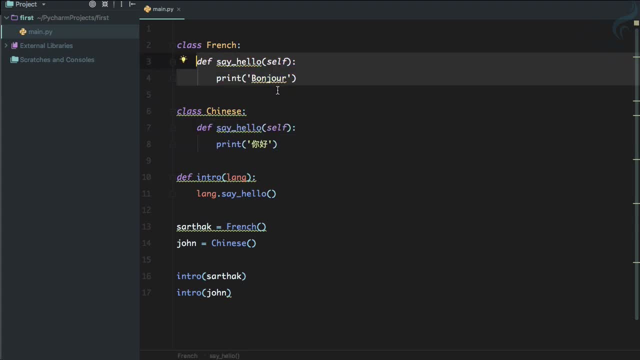 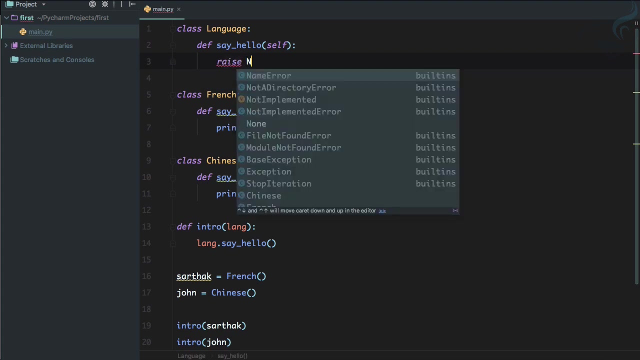 of same function for different situations and sometimes what you do, you can define an abstract class. so I will say class of language and this is going to have a same function called say hello function, and this is not going to implement anything and it's just going to say not implemented. 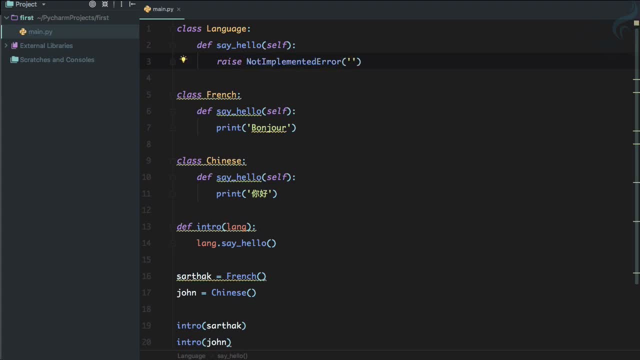 error? this one, and the error is: please, uh, use say hello- class in child class. okay, so this is the class I have created and it's a abstract class because this function is not doing anything, just raising the error, and now i can easily use the inheritance and extend. 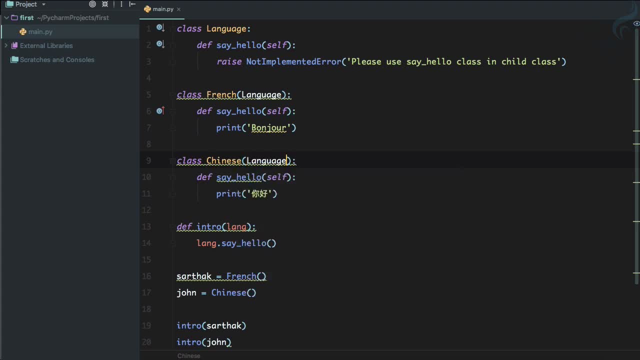 this class or use this class for both of the languages. and now if i run, there is no effect on that, but if i somehow remove this- suppose i don't have the french say hello function. what it's going to do? yeah, it's going to call this function and you can see it says some error.